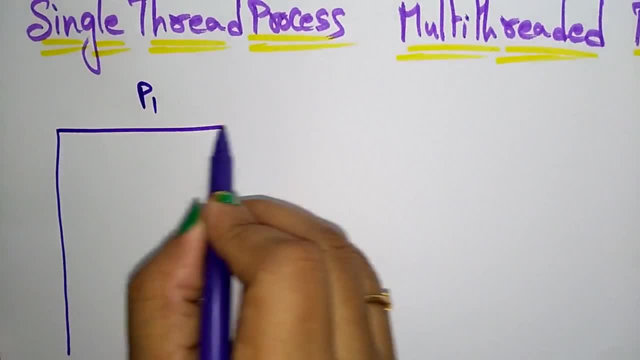 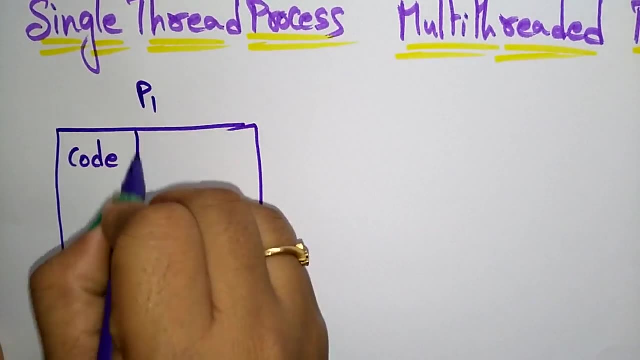 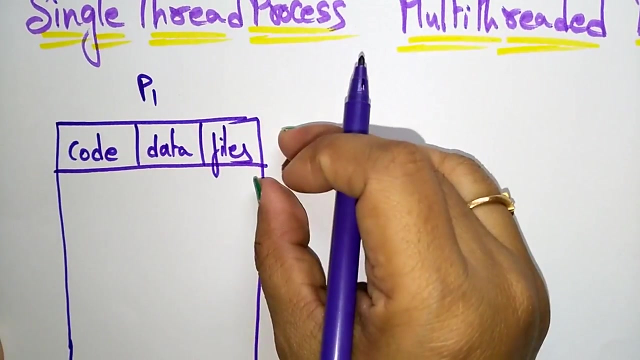 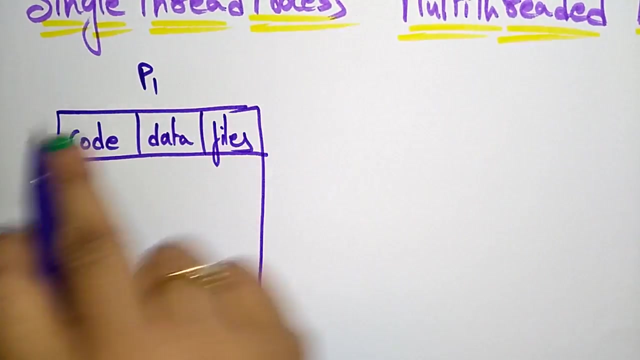 Okay, The working of a single thread is like this. Okay, So here the code data and the files section will be there. So these code data files will be shared by all the threads. So if it is a single thread, that will be shared. If you are having a multiple thread, that will be shares the common data and common code and the common files and coming. 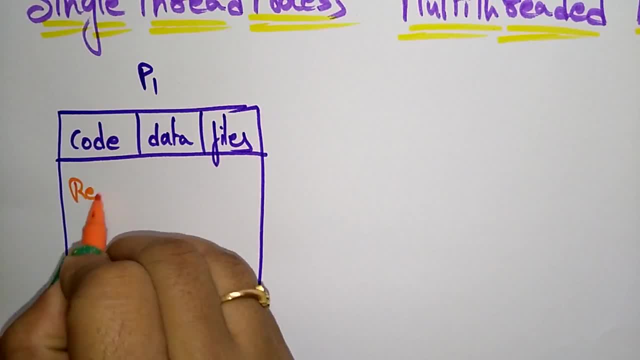 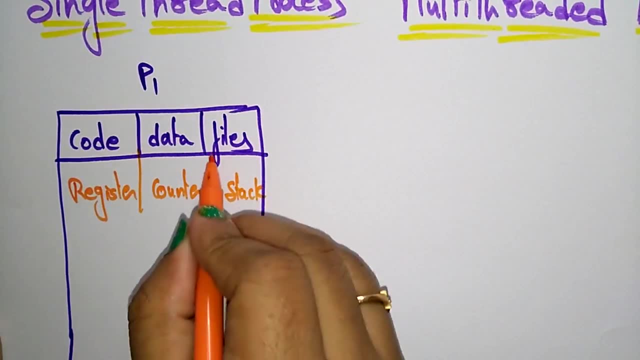 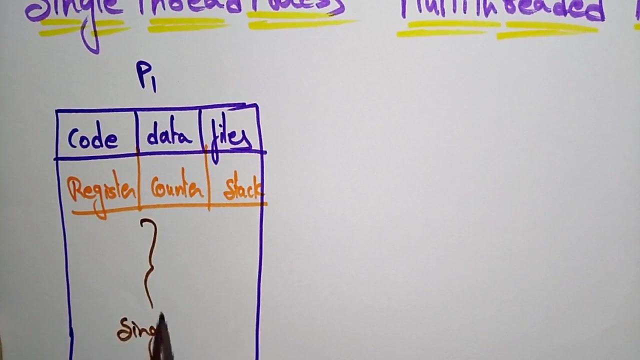 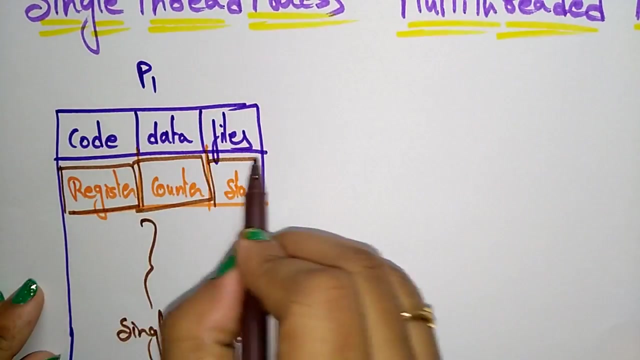 to the single thread thread, you are having only one register program, counter and single stack. so if you are dealing with only but single thread, if only if a process is having only a single task, a single thread, that single thread is having only register program, counter and the stack. so I already explained the definition. so 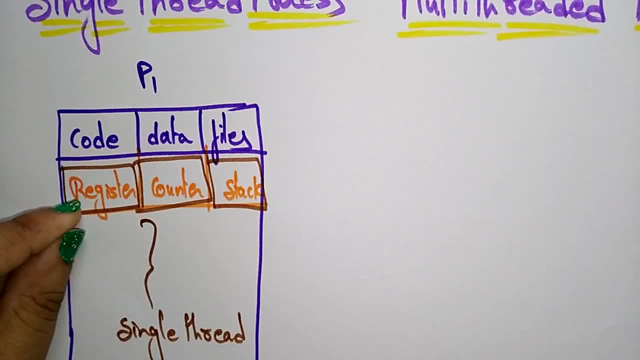 whatever the thread is there. so that thread is having the register to store the data and the counter is to program. counter contains the next instruction that has to be executed. that address will be store. next thread address will be stored in counter and the stack contains the temporary data. so next what? 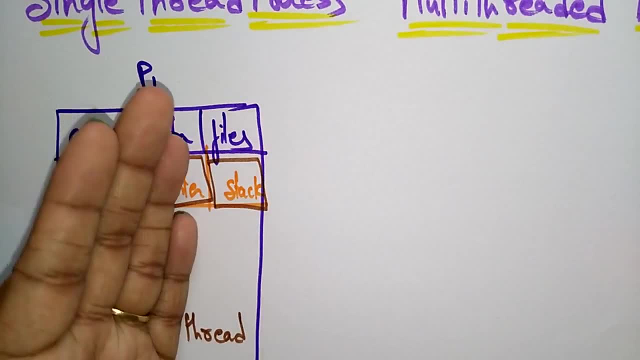 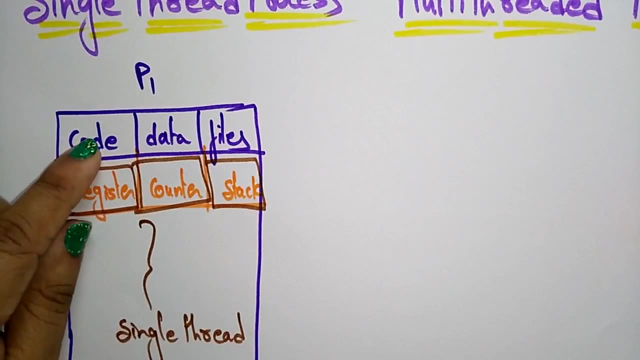 data has to be executed means first in, like that stack operation, the top has to be deleted, like that. so all these register counter stack will share the code data and files that are present in the process control block. so this is a process control block which in the process control book you are having the 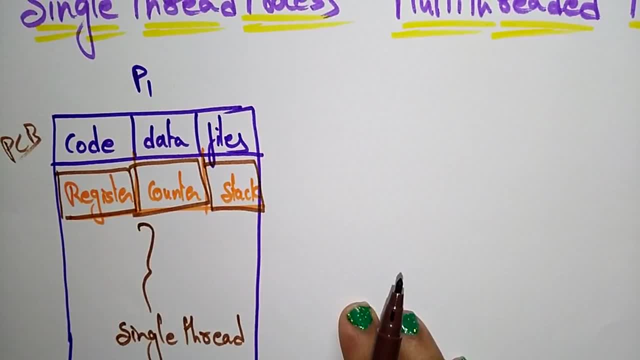 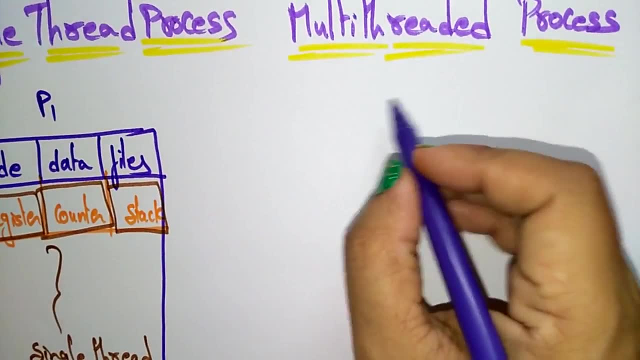 code, data and the files, and that will be shared by a single thread. so this is a single thread process. now let us see the multi thread process. what is this multi thread process? let us take P 2, so let's take the P 1 only. process P 1 and. 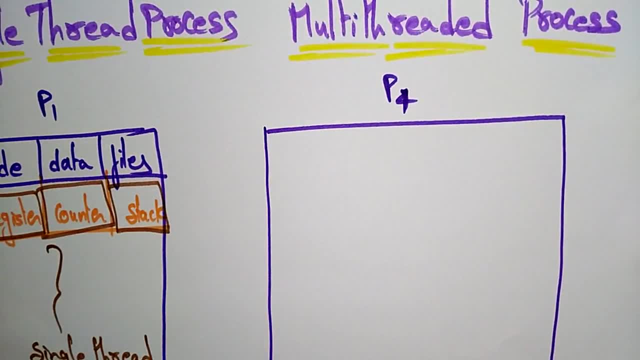 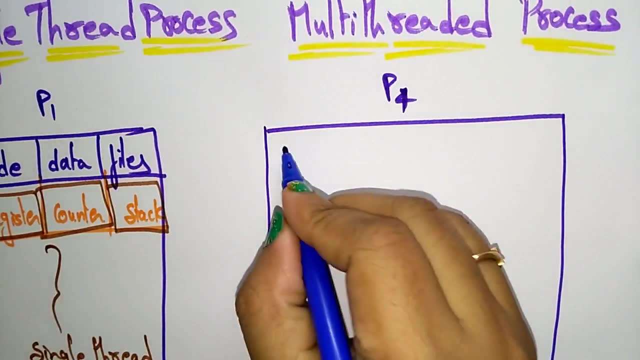 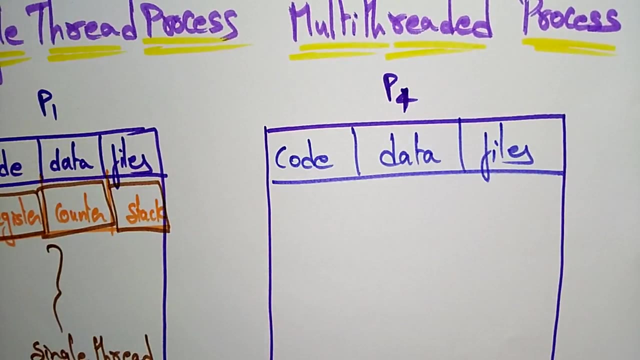 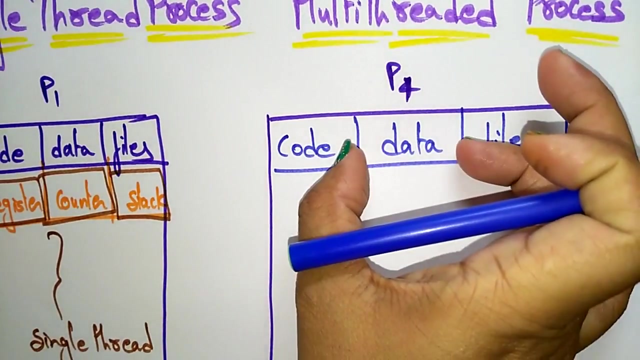 P 2. so a single process. so this is a single process. this process is having same like code data and the files. so the only this process control block will store the related process information, code data and the files, and this information will be shared by all the threads. so here you are having, suppose, the